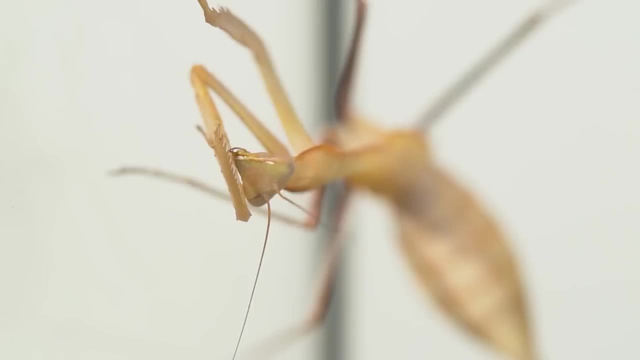 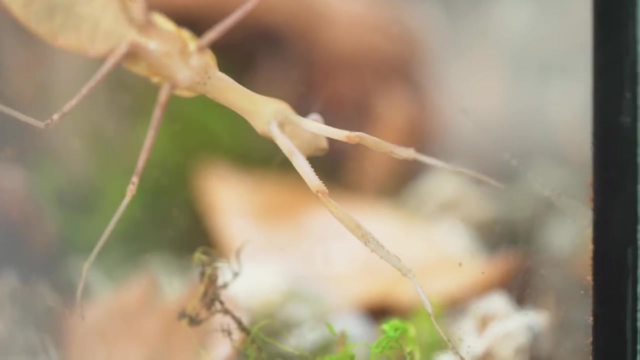 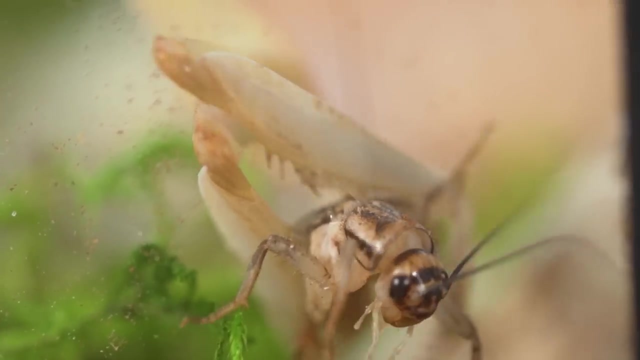 But Bertschrude wasn't the only thing alive in this enclosure, As just earlier I had put a couple crickets inside, Immediately after Bertschrude sensed them and rushed in towards the prey with killer instincts. Seconds later, the cricket was now getting crushed by Bertschrude's claws and ripped. 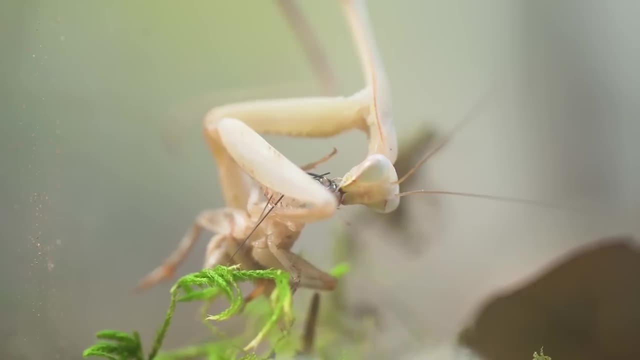 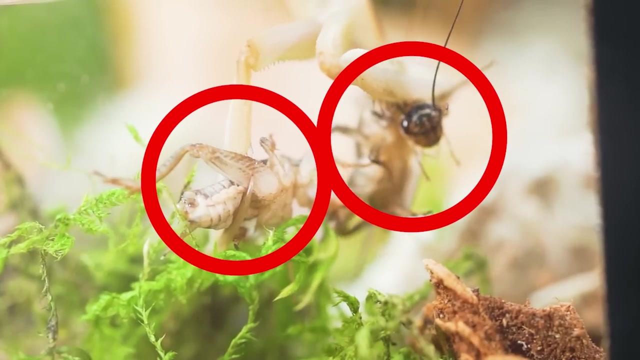 apart by her alien mouth. But whilst the mantis was enjoying her meal, another cricket walked by, So she snatched that up and started to eat two crickets at once. Clearly she was pretty hungry. Now Bertschrude was hungry, so she started to eat two crickets at once. 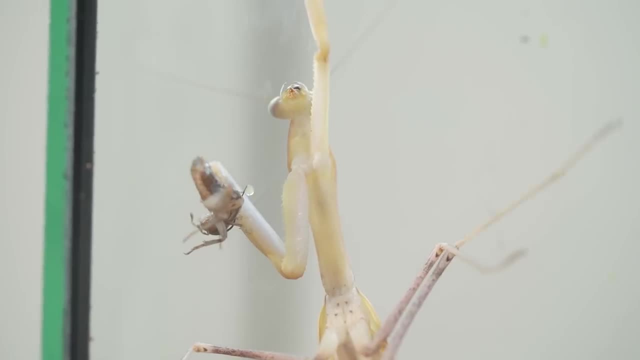 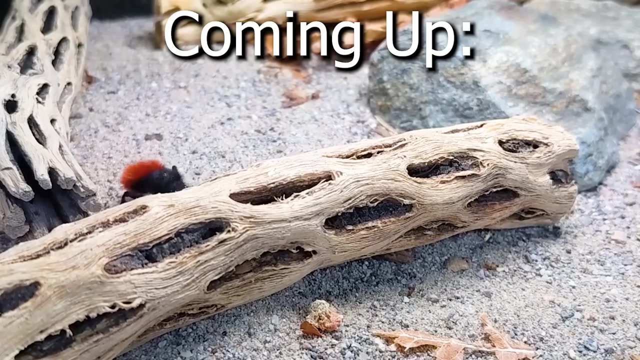 Now Bertschrude has got to be one of the coolest insects I've ever seen. Like seriously she looks like King Kong right now. But there are still six more insane insect species I'm going to be showing off in this video, including a cow killer that is known to have one of the 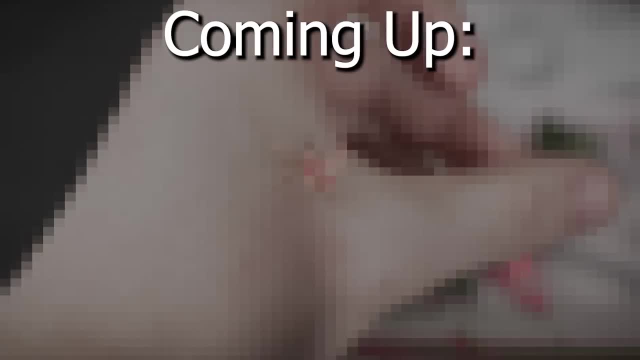 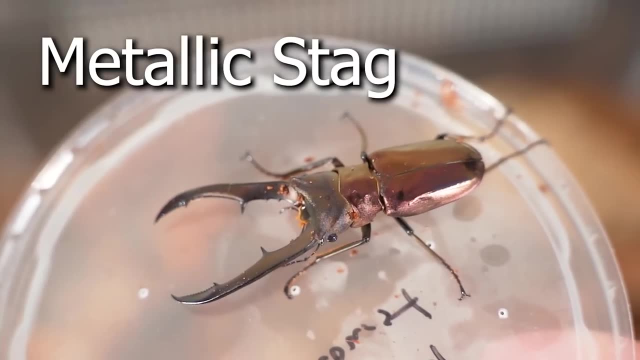 most painful stings in the entire world, And I'm going to be holding it. Yeah, But before getting to the cow killer, let's say hello to insect number two, a metallic stag beetle. Now, this is straight up an exotic insect. I mean, it literally looks like it's from the future. 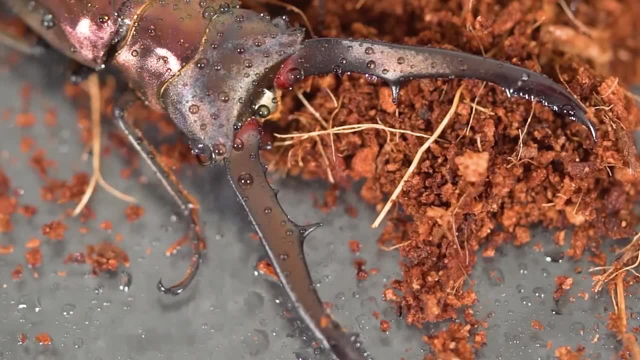 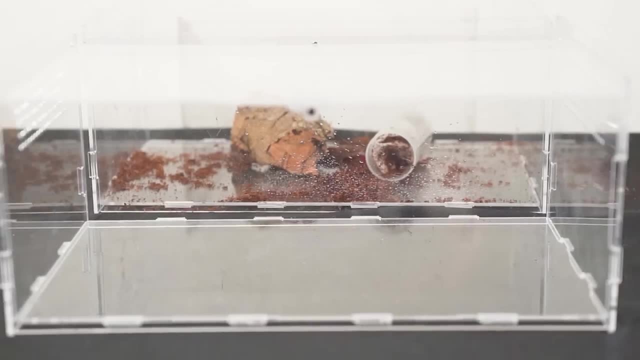 This species has some of the largest mandibles out of any beetle species And, honestly, those big, sharp mandibles make me too scared to pick it up, So instead I just picked it up with this plastic lid For its enclosure. I'm using this 14 by 8 inch tank And watch this When I 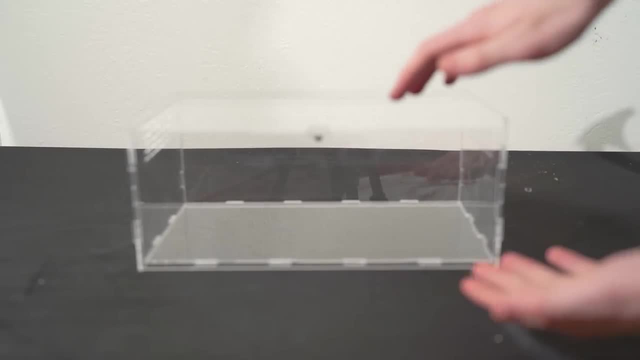 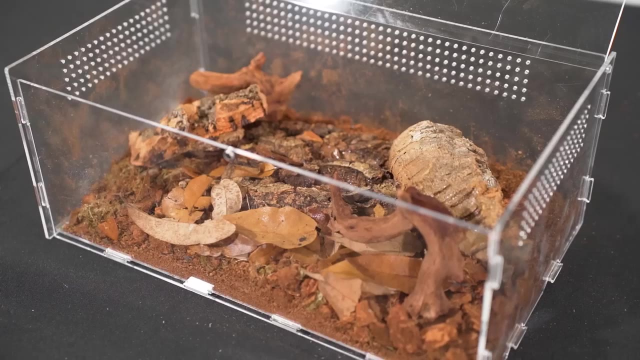 clap my hands in front of the terrarium, it's going to be instantly built. Three, two, one, boom. Now that's a super clean transition. As you can see, there's tons of stuff in here, like bark and sphagnum moss, that will be perfect for the beetle to hide under. And speaking of the 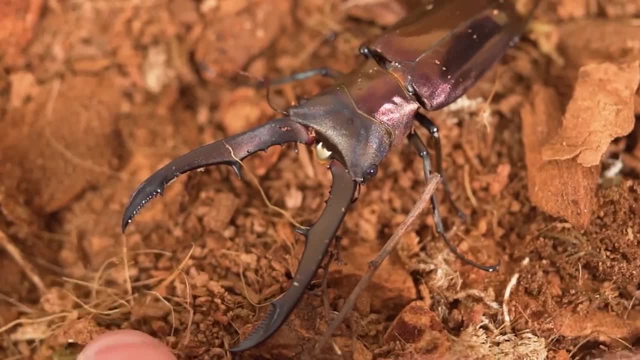 beetle. I have a lot of stuff in here. I have a lot of stuff in here. I have a lot of stuff in here. I of course need to give this guy a name And, since you know, it's the best and coolest beetle. 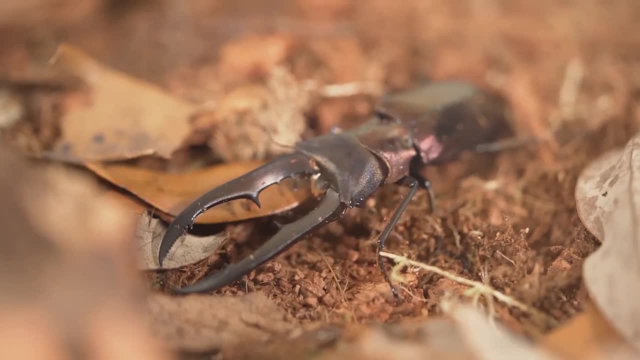 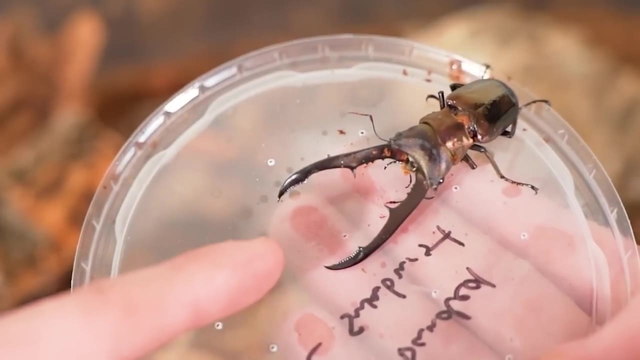 ever. I'm going to name him Paul McCartney Because, you know, I just feel like that name fits him pretty well. You know, he looks like a Paul. Anyways, despite Paul having these absolutely massive mandibles, he doesn't even use them to eat prey, because he's a boring herbivore. 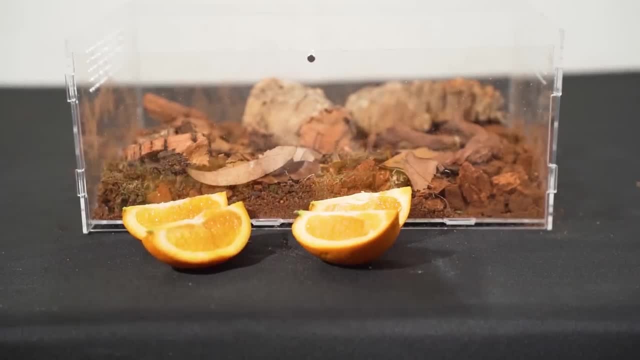 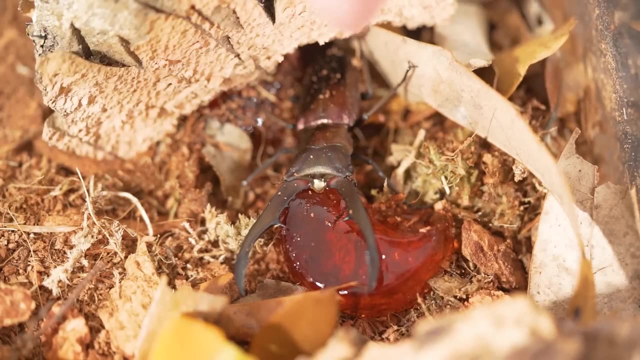 So to feed him, I just got an orange and put it inside. I also put some of this beetle jelly because I think they like eating this too. But Paul is a male beetle and he looks pretty lonely. If I were to name him, I would name him Paul McCartney, And I would name him Paul McCartney. 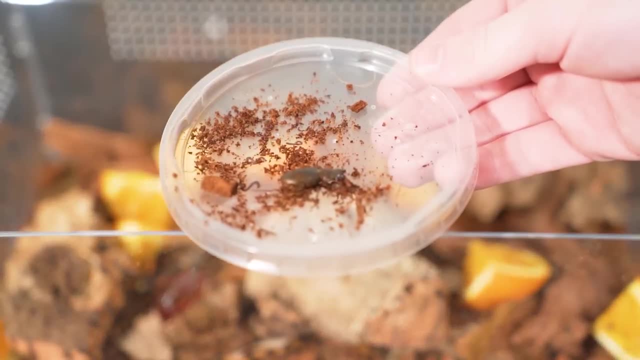 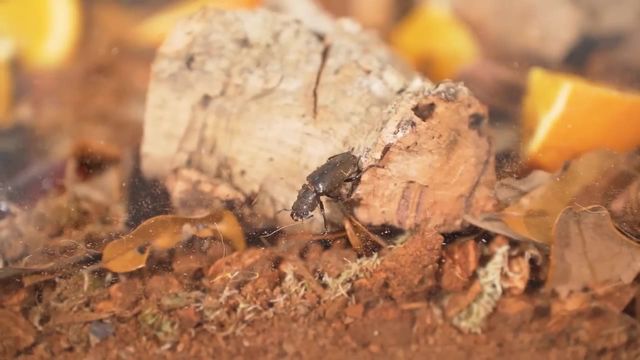 If I'm being honest. So I also got this female of the same species. that is honestly a lot uglier than Paul, because she doesn't even have those cool mandibles. But I put her in anyways And soon she started to wander around. Eventually she even climbed onto Paul's back while he was. 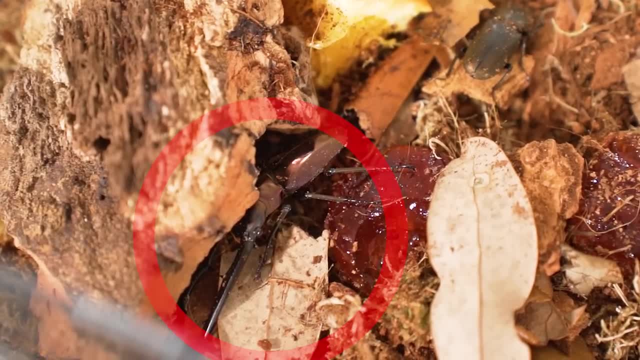 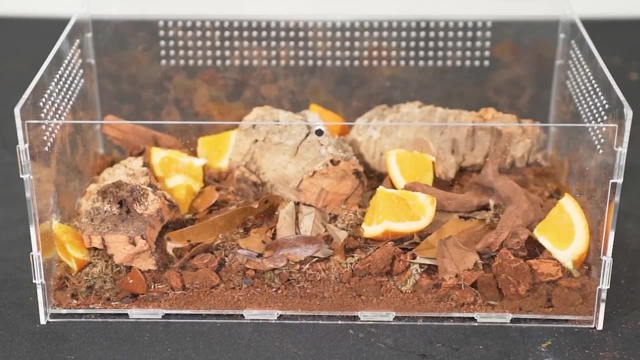 sleeping, which seemed to annoy him, And he got up and walked away. Not a great start to these beetles relationship, but I'm sure Paul and this new female will eventually enjoy their home together and might even have little beetle babies. And remember, later I'm going to be picking up a. 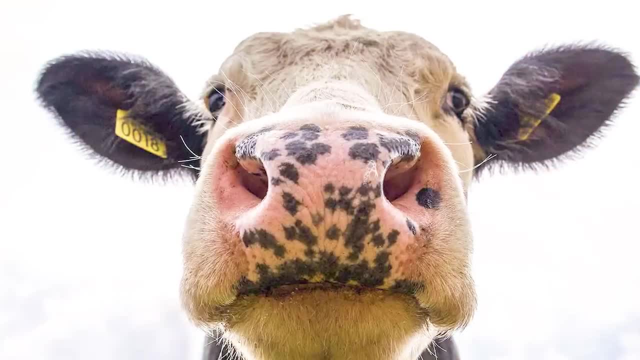 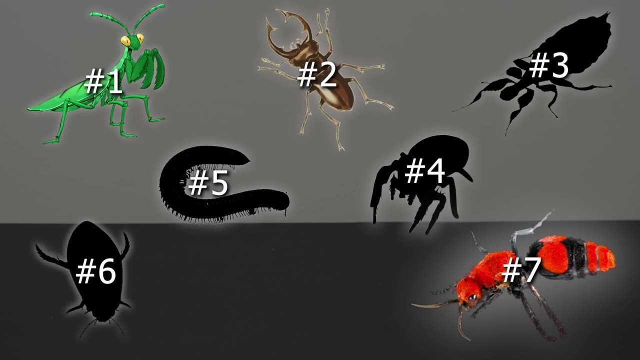 cow killer wasp, which is said to have a sting strong enough to kill a literal cow. I hope it doesn't sting me. Anyways, as you know, we still have more exotic insects to showcase And for this next insects, let's play a little game When I move my camera down. 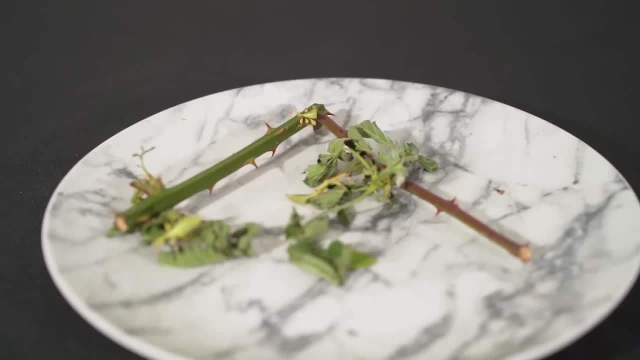 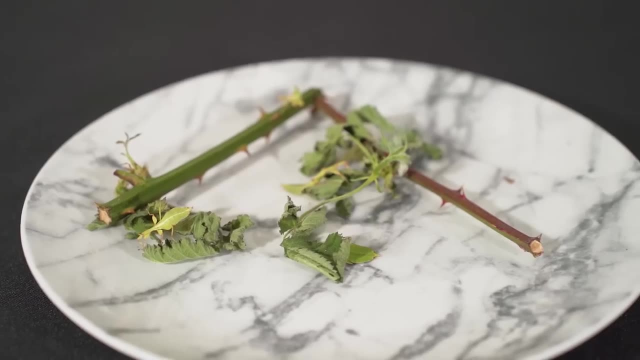 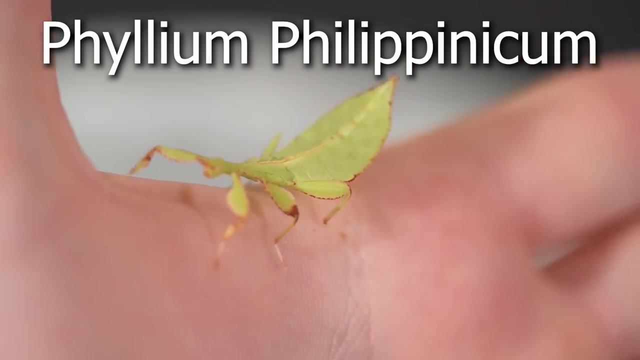 you have three seconds to find the insect in the frame, Let's go. And did you find it? Well, probably not, because this insect actually has a very special disguise scattered around here. It's a species of insect called philium Um, commonly known as leaf insects. Anyways, I don't have much to say about these guys, I just 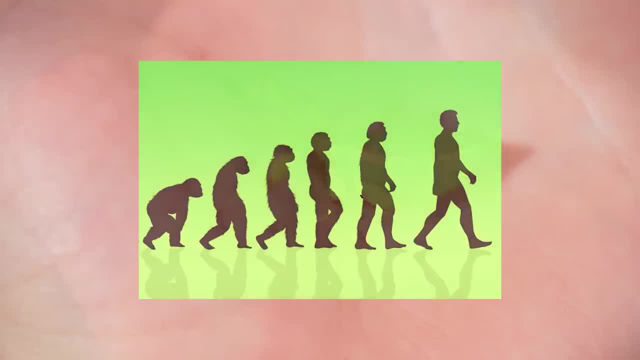 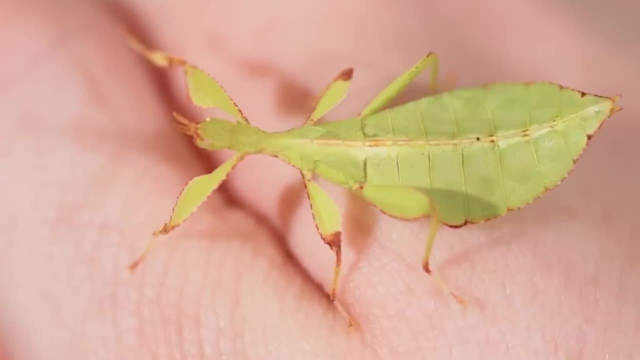 think it's pretty funny how, over millions of years, they've evolved to look like a leaf. I mean they could have evolved to have huge teeth and claws and stingers, but no, they evolved to look like a leaf. Now for their home, I got this glass terrarium. That's a bit. 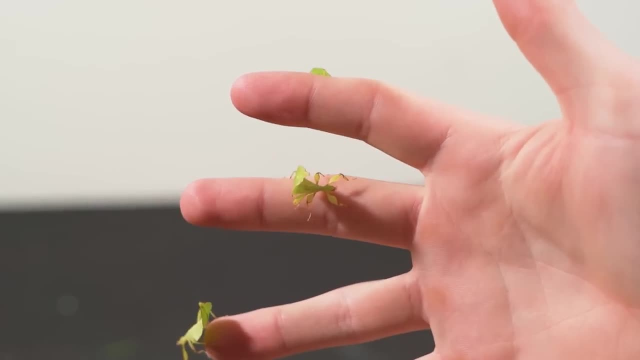 bigger, since we had four of these bad boys, which will all eventually grow to be about five times as big. So I needed a lot of space. I wanted to make this look like a plane's biome, So I got some of these bad boys. I got some of these bad boys. I got some of these bad boys. I got some of. 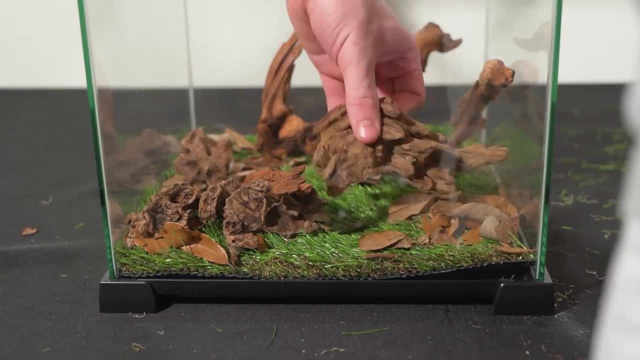 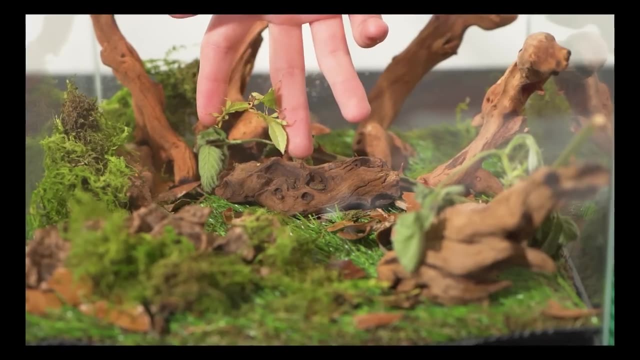 some artificial grass And I also put a bunch of tree branches all around the tank, So the leaf insects could pretend to be leaves, just like they were born to do. Welcome to your new home. boys, I hope you like it, or girls- I don't know if they're a boys or girls- that most of the little leaves. were just walking around and enjoying themselves, But a couple of the leaf insects started praising to the gods or something by raising their hands in the air and doing some sort of ritual. Anyways, these guys diet consists mostly of themselves, And by that I mean they eat. 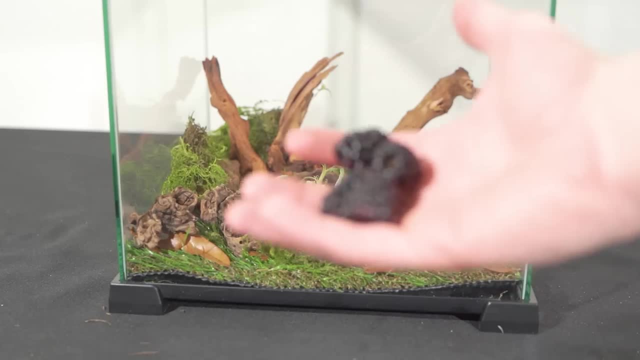 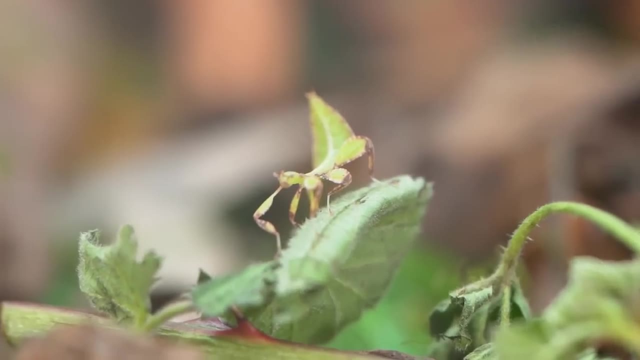 leaves. So, yeah, they're basically cannibals, But their absolute favorite food is blackberries, So of course I put some of those around the tank. Well, this is pretty good. I think these leaves are going to live a fantastical life in here. Moving on to the fourth insect, we got a fierce 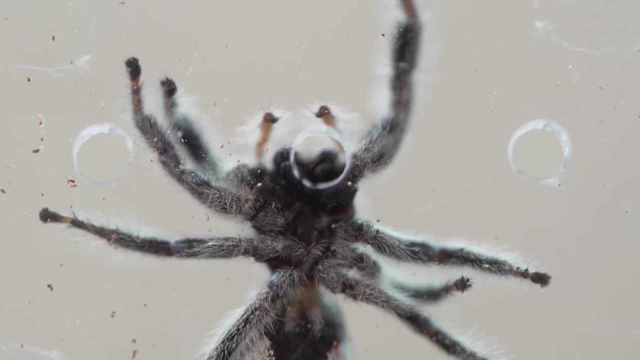 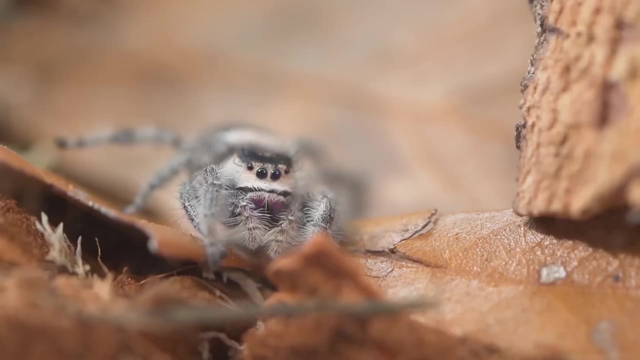 apex predator. Not only does this insect have fangs, but he also injects a potent venom into anything it bites. Everyone say hello to one of my jumping spiders. Now, yes, technically, by definition, this isn't an insect, But by my definition of an insect, it is. 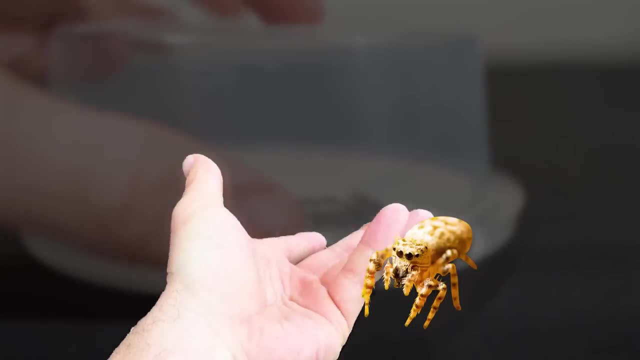 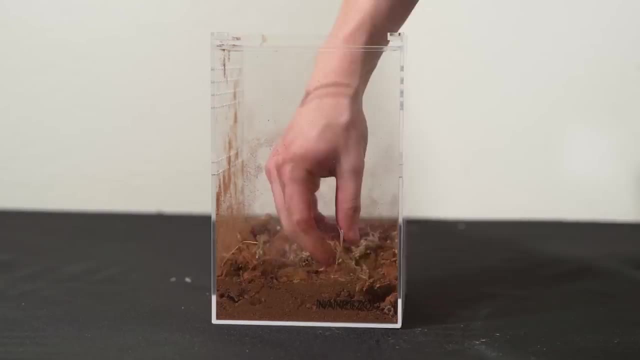 So don't comment about it. Now I'm not going to pick up this guy with my hands, because they're super fast and he'd probably just jump off my hand and go hide under the couch or something, And I don't want that. So I'm just going to speed run his new home real quick with tons of places. 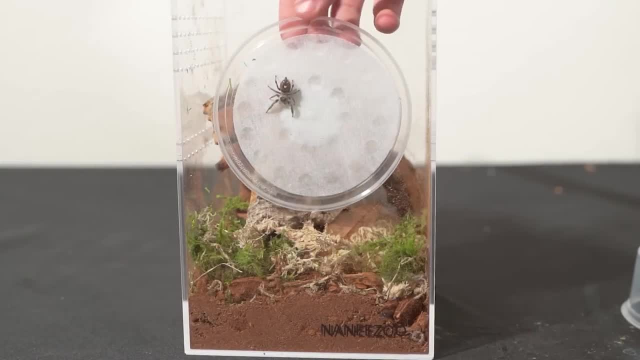 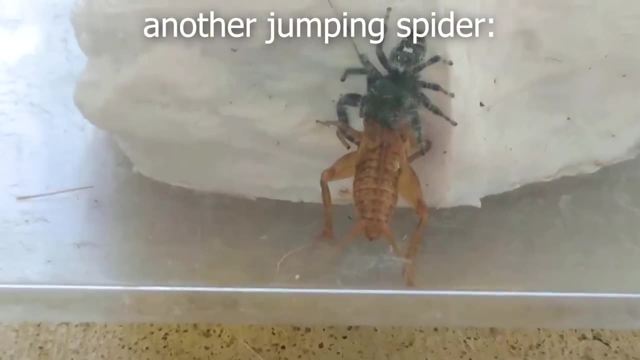 for him to jump around And boom, let's get this little guy into here. These spiders are actually one of the coolest species, because most of them have the ability to eat prey up to three times their own size. So of course I had to challenge my jumping spider by dropping in a few pretty 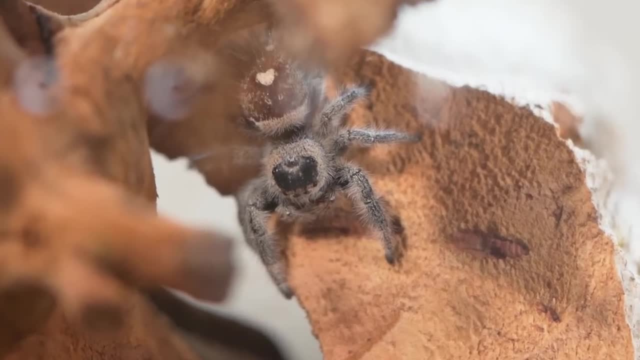 decently sized crickets. So I'm going to try and challenge this guy And I'm going to try and try and challenge this guy, And I'm going to try and challenge this guy, And I'm going to try. and immediately, the jumping spider hit on this piece of wood, seemingly waiting for the perfect moment. 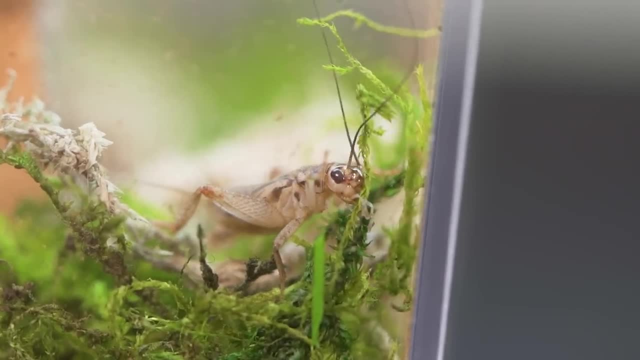 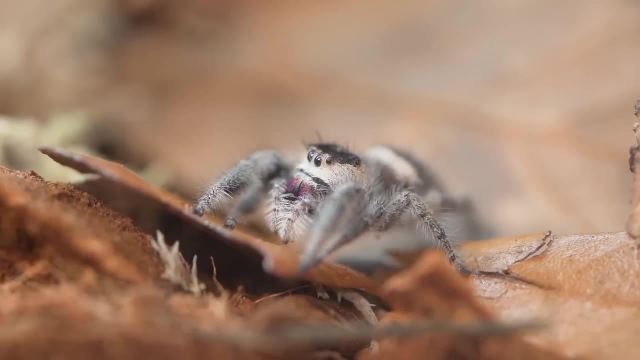 to strike a cricket, But the funny thing was that he never actually did any attacking. If anything, the jumping spider was actually afraid of the crickets because every time he saw one he got startled and slowly walked backwards. It was actually pretty funny. 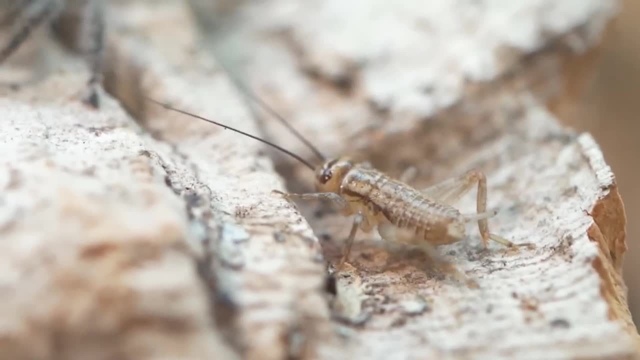 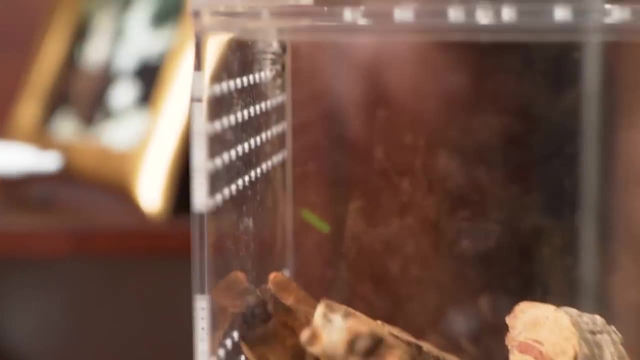 So to feed him, I got a couple of smaller crickets and put those inside, hoping he would eat those, But it kind of still seemed like he was scared of those as well. Well, I guess this guy's just not hungry right now. So in the future, if he still doesn't eat any crickets, 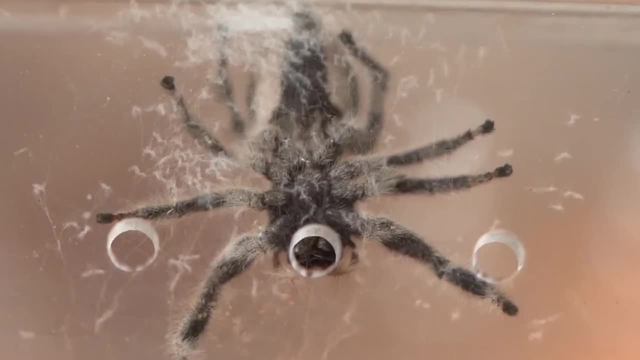 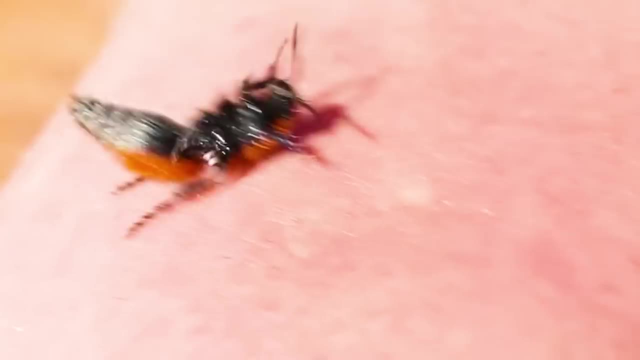 I'll try feeding him some smaller worms and stuff, But for now let's move on. I've been saving the best insects for last, and coming up soon I'll be holding the cow killer wasp, which of course is the deadliest insect out of all of them. But first for insect number five, let's play another game. 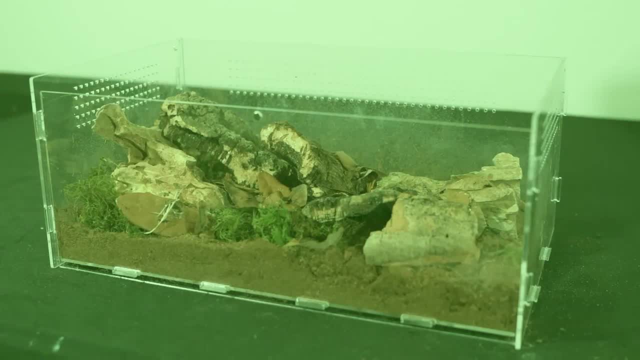 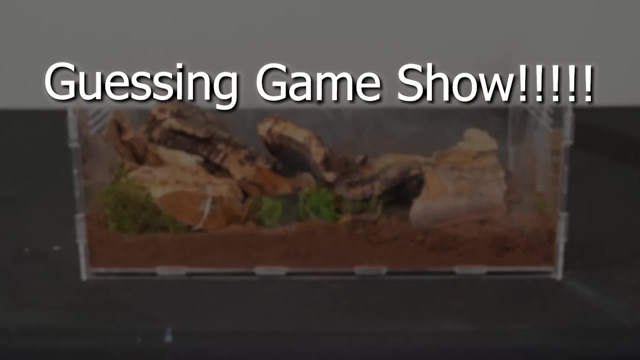 I'm going to build this enclosure just like this And, as you can see, I built a nice little dirt enclosure with wood and moss. So now can you guess what I'm going to put in here, based off of the enclosure? Your options are A- a shark, B- a dog, or C- an earthworm. The answer is: if you guessed. 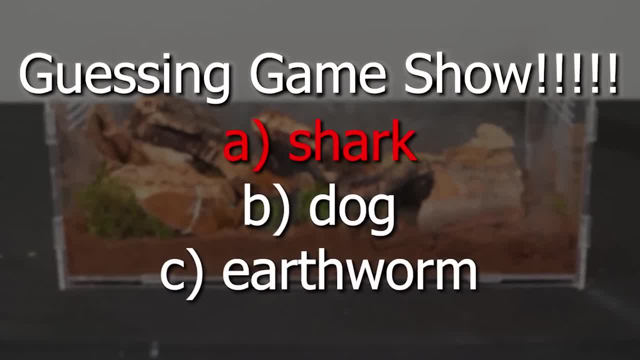 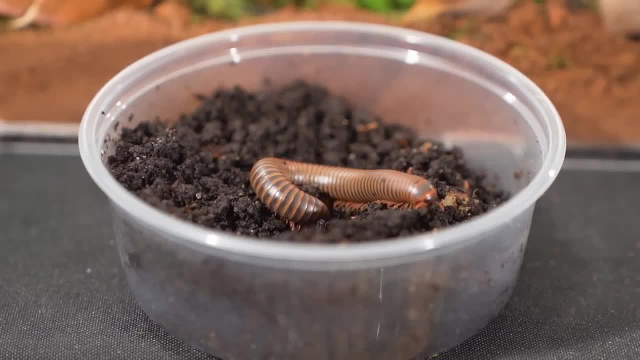 shark, you were actually wrong. The actual answer is: none of these. It's D a millipede. And yeah, technically, once again, this isn't an insect, but don't worry about it. This species in specific is a pink-toed millipede, which, to be honest, I don't know why it's called that, because its toes. 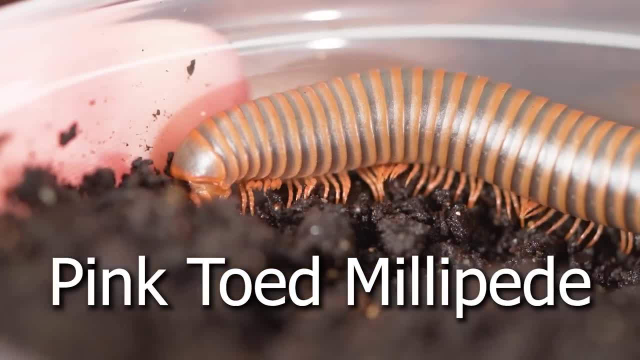 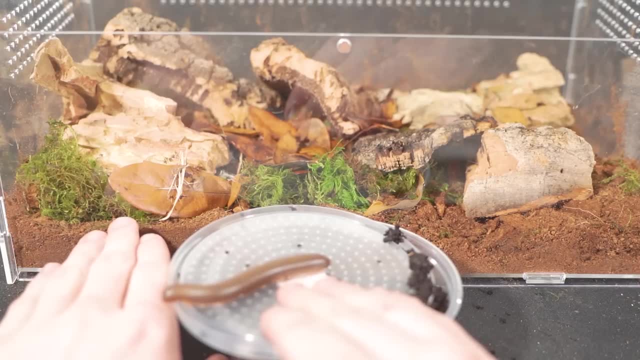 are not pink, I mean, it doesn't even have toes. If anything, it should be called a orange leg millipede. but whatever, Despite it being kind of disgusting looking, I built up enough courage to pick it up onto my arm. 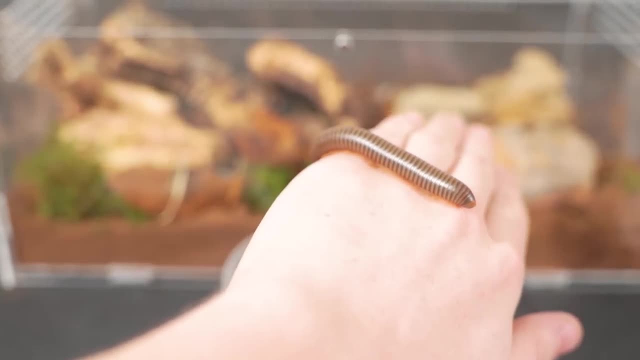 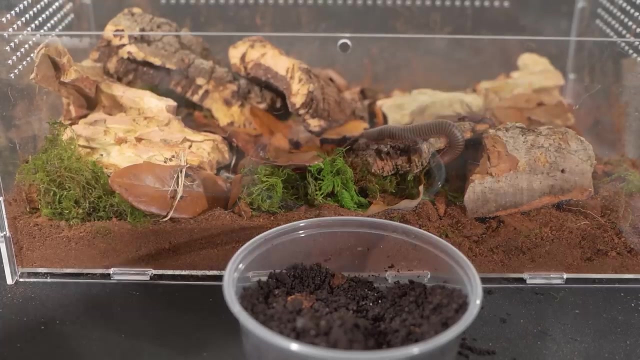 and move it into its enclosure. Oh, nah, this feels so weird crawling on me. What the heck- I swear this is actually like stinging me right now. What the heck This feels so weird? Yeah, get off of me. You see, millipedes have hundreds of legs, which helps them grip on to stuff and 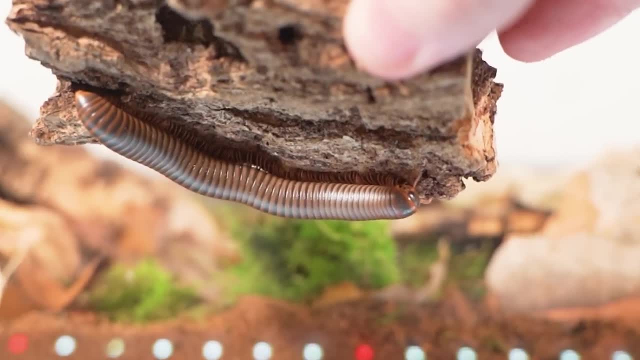 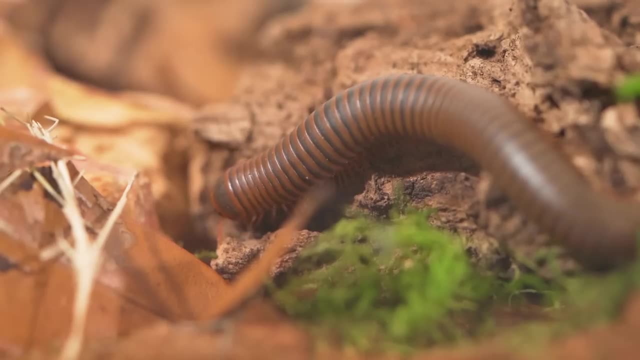 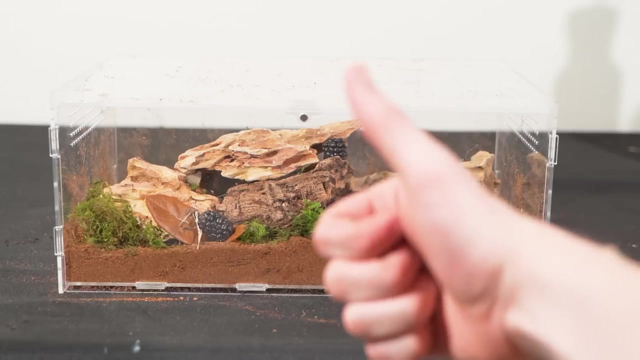 allows them to even walk upside down. Okay, maybe it's not that cool. Now, unfortunately for this, ever and basically just only eat decaying matter. So I'm just going to put some blackberries in here and, yeah, call it a day. Enjoy your home, little guy. Now for insect number six, which actually 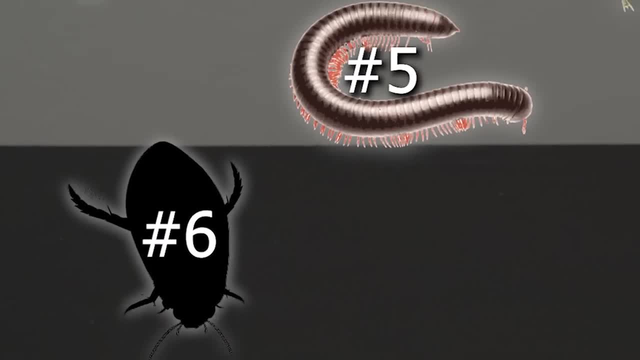 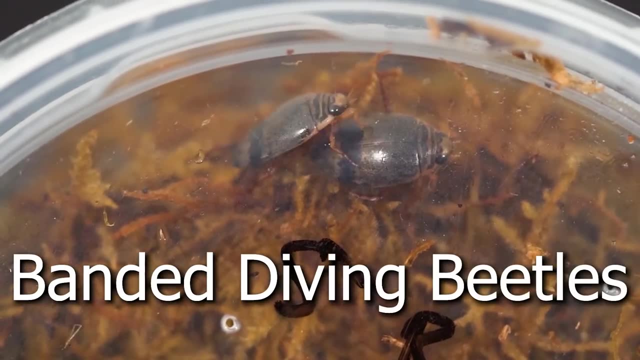 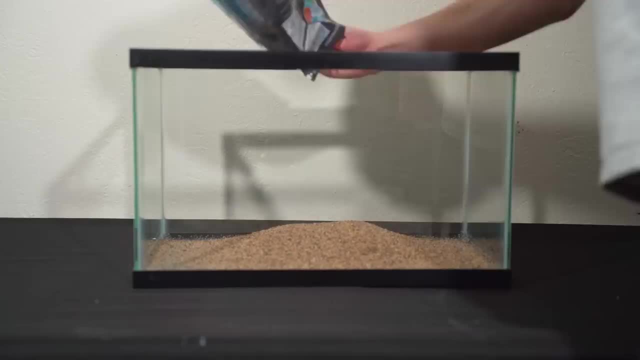 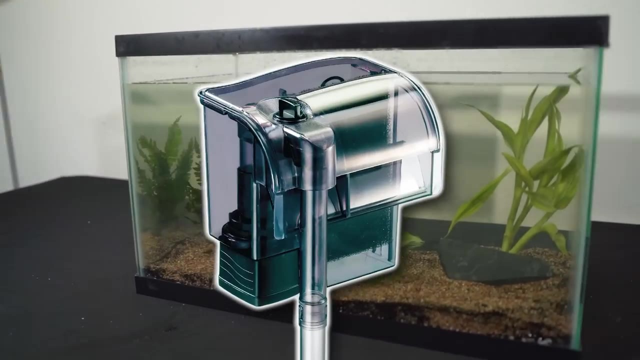 I got this 10 gallon aquarium And basically I'm just going to fill it up with substrate, aquatic plants and, finally, some water. Now, the best things about these guys is that they don't even need a water filter, since they are much less affected by variability in nitrogen or 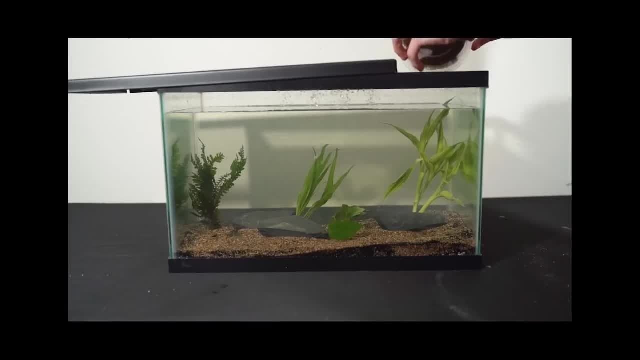 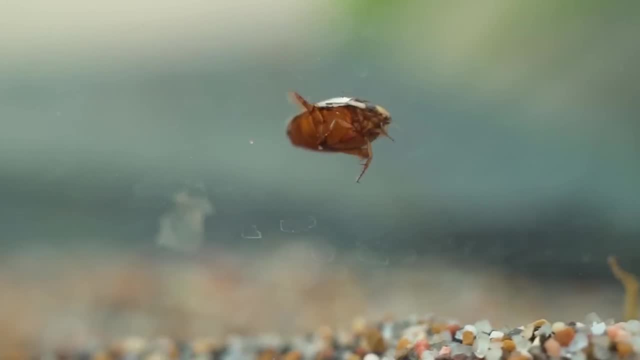 phosphorus concentration because they do not breathe. So yeah, let's put them in. The little beetles were shy to come out at first, but eventually the tank was swarming with all seven of them. The way they swim is honestly just really cool, because they got these little. 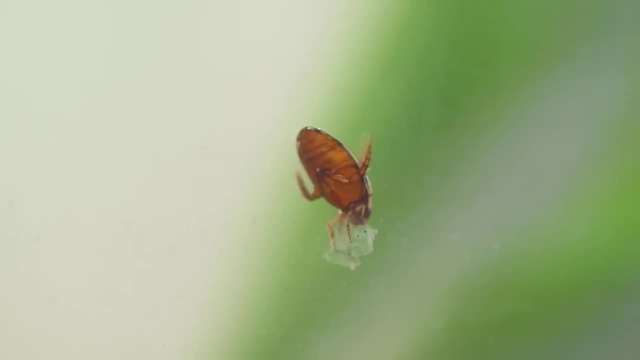 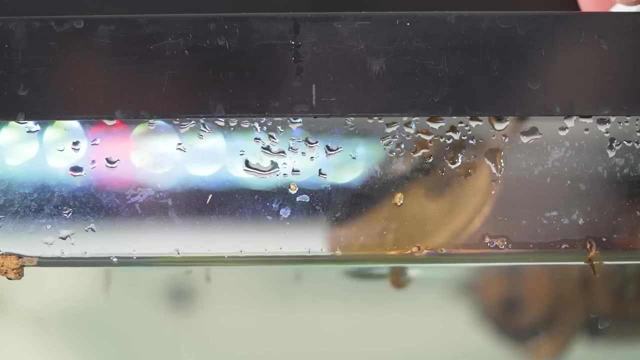 legs and stuff that they propel themselves with, which I guess is just kind of normal and not that cool. But now I want to show you guys how these beetles eat prey. So to do that, I got some meal worms and dropped them in the water. After a few minutes, amazingly, a beetle stumbled across a. 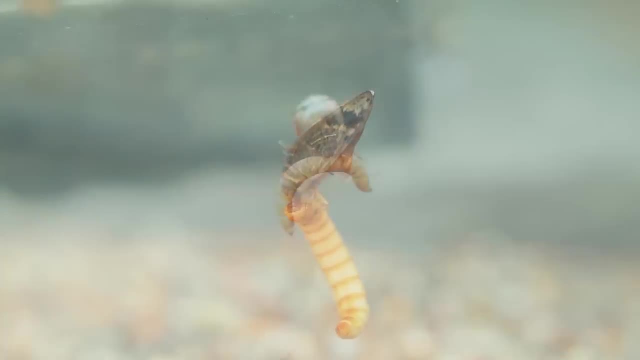 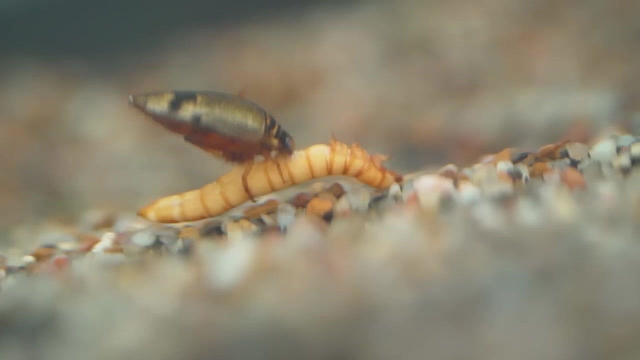 worm. So he grabbed it with his legs and pulled it all the way up to the surface of the water. When he got there, he started to absolutely devour the meal worm by sucking the life out of it. A couple more of the aquatic beetles found some more meal worms, So soon enough. 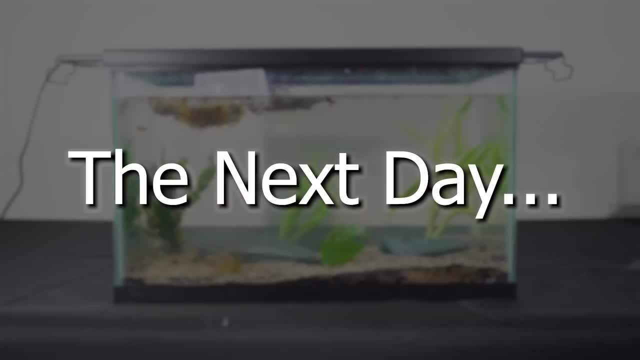 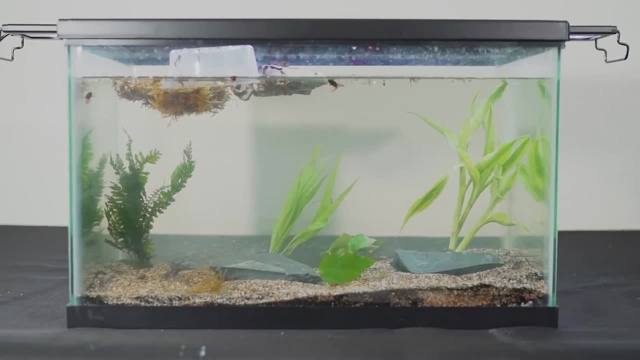 the entire tank was feeding on these guys. The next day, I came back to find these little lifeless meal worm exoskeletons laying around the floor. Clearly, the beetles had enjoyed their meals. Now, this is the moment we have all been waiting for: The seventh insect, a cow killer. Well, 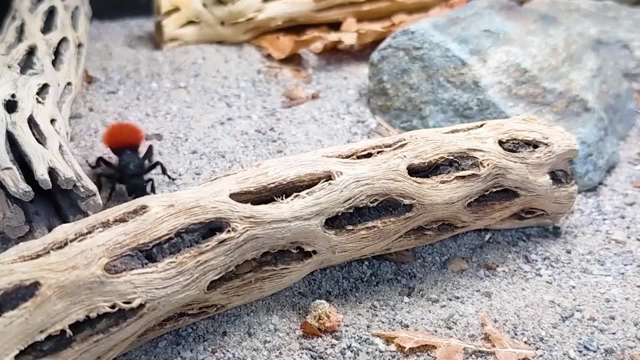 this is just a box, but inside of it, the cow killer awaits. Now, the actual name of this is a velvet ant, but it's not a velvet ant. It's a velvet ant. It's a velvet ant. It's a velvet ant. 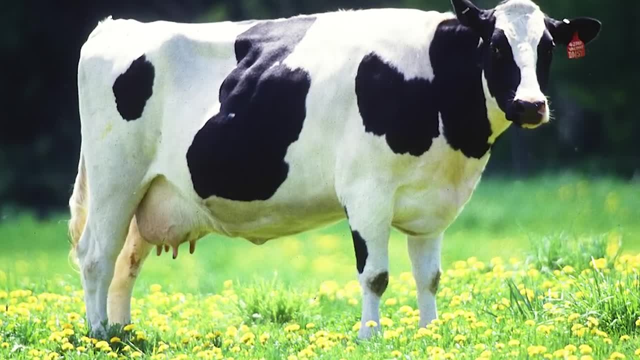 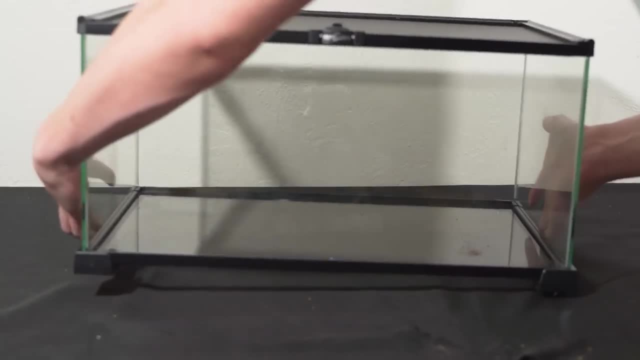 But the legend has it that its sting is strong enough to kill a literal cow, Hence why people call it the cow killer. And I'm about to have it crawl on my bare skin. But before that I need to have its enclosure finished. 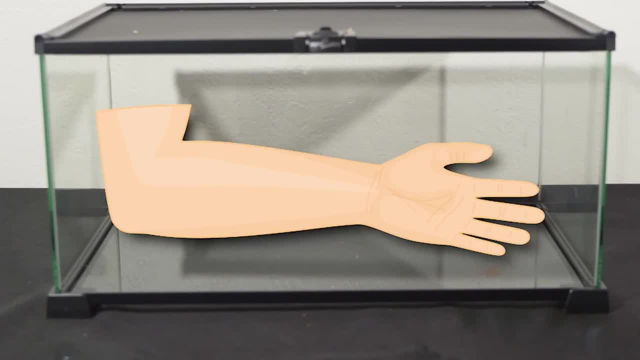 So I have a place to you know put it, so it's not just stuck crawling on my arm. These guys live in the deserts, in the wild, So I'm going to quickly recreate that here by doing another super cool transition. Watch this. 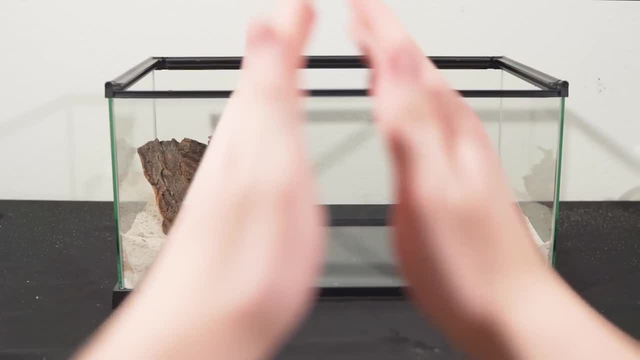 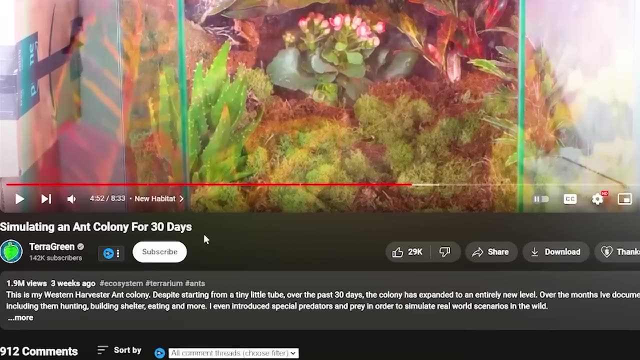 As I squeeze my hands in, the desert magically appears: Wow, Okay, now that's actually a super cool transition That deserves a subscribe. Seriously, subscribe. Scroll down right now and click subscribe. Please, I am begging you. As you can see, I got a heat lamp to make this place nice and hot. 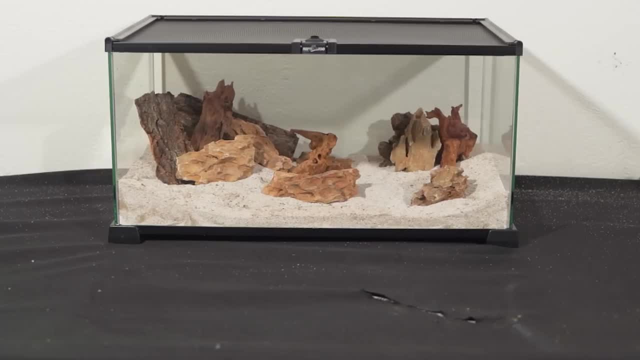 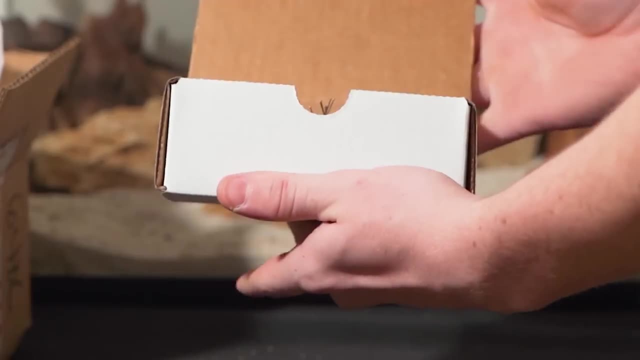 And also lots of little places for the cow killer to hide under. Speaking of the cow killer, I should probably stop stalling and just get to opening it up. So I opened up the box and apparently I accidentally bought a dead taxidermied cow killer and not a real, alive one. So, of course, I went to buy an actual, alive one online And unfortunately, I found out that you can only get one when they're in season, Through July to August, And since it's April right now, I found out that it's literally impossible to get a cow killer now.